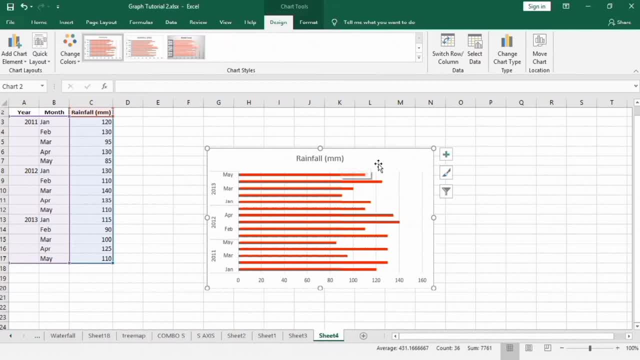 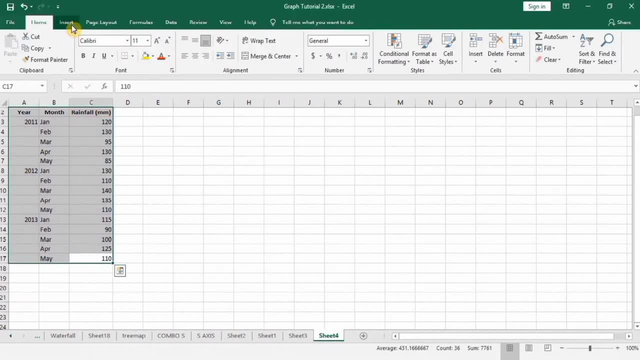 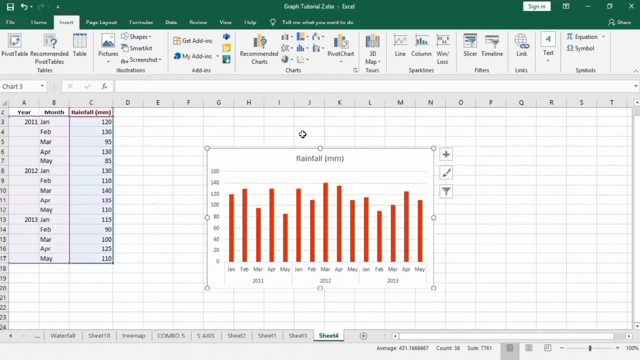 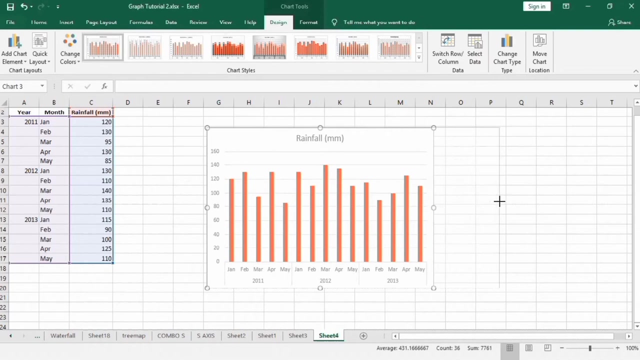 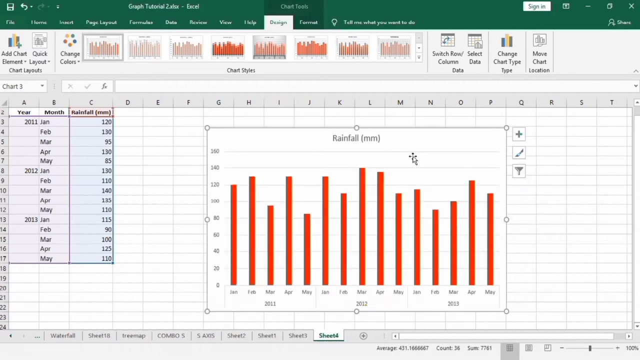 so your graph will appear like this, but I will proceed with column graph. So I will insert column graph. Go to here, and here you will find the option of clustered column chart. Then resize it. Now I will insert the title here: Put equal sign in formula bar. 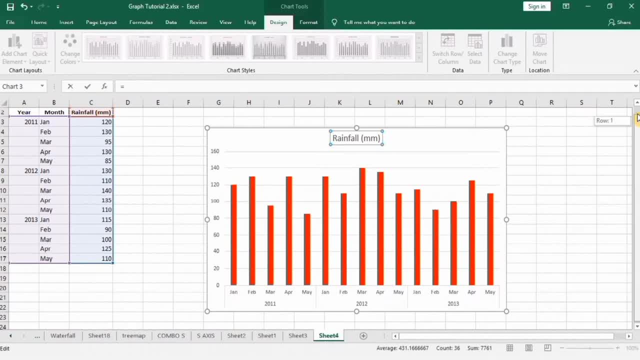 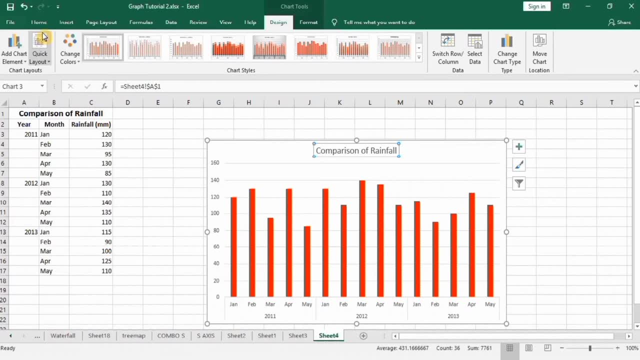 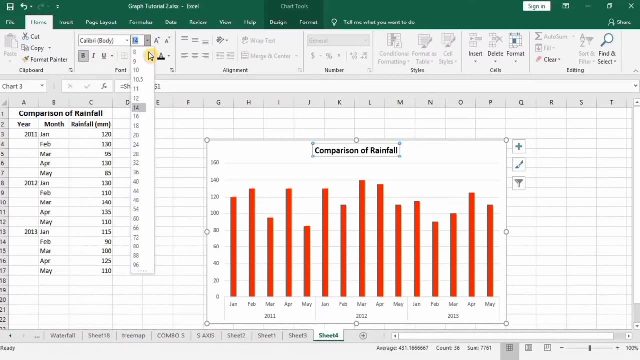 and select title. If you have right here, press enter, Go to home and adjust it font size and color. Now I want to remove these grid lines, Press this positive sign and uncheck this, and I want to insert axis. So I will go to this option and only y axis. So press this arrow and primary vertically. 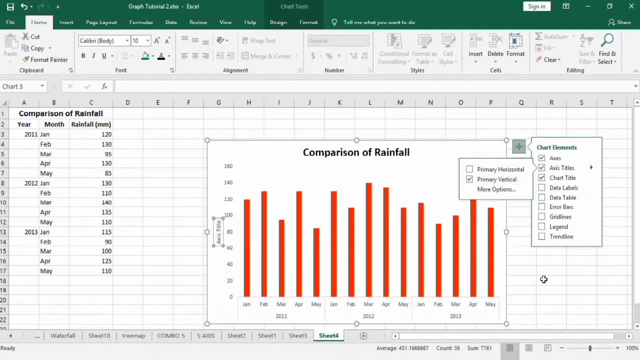 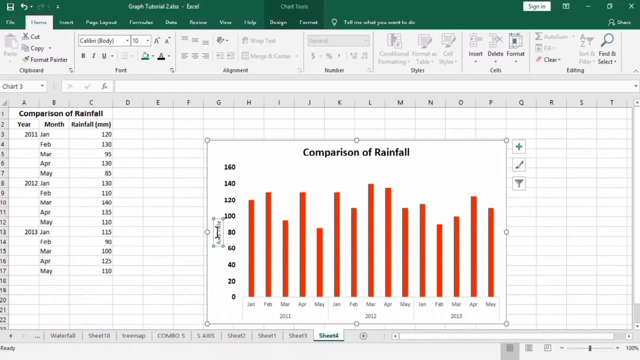 check this option. Now I will format these axes. I will change the size of the axis. So I will change the size of the axis to 12, and 12 with black color. Similarly, I will change its label. Put equal sign by following similar step as we follow in title. 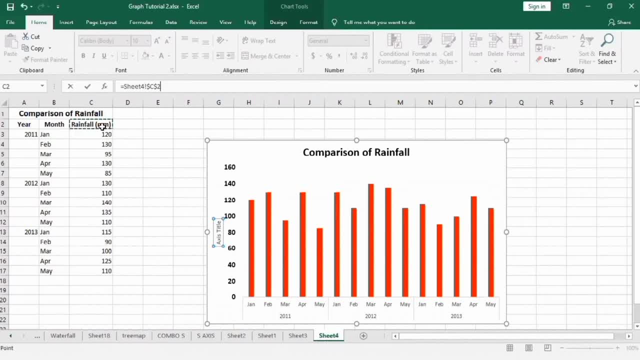 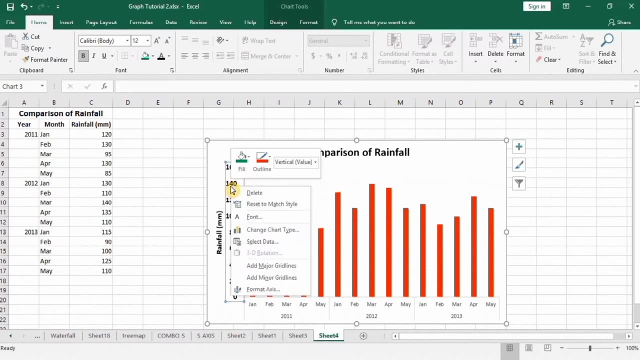 Press enter. Now I will change the size of the axis. So I will change the size of the axis. So I will change the size of the axis Now I will change the size of the axis to 12.. Now select this Right click if you want solid line on axis. 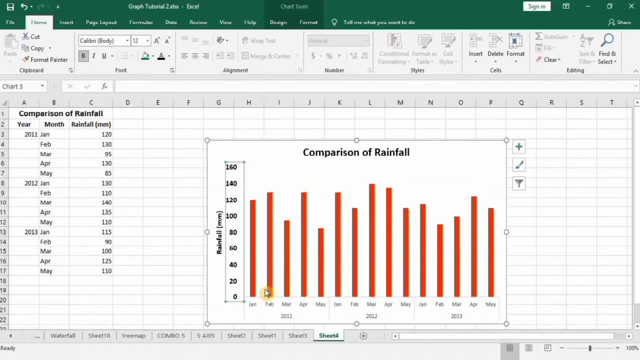 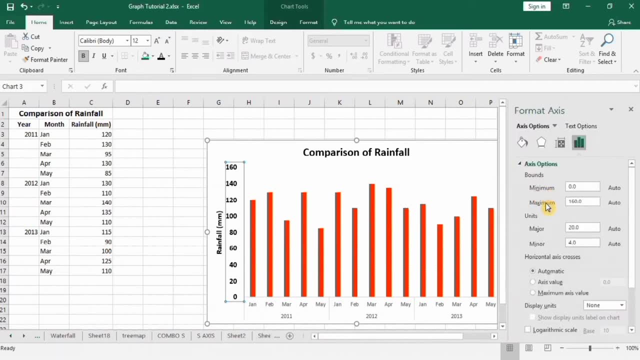 and tick marks. Go to format axis. From here you can adjust the minimum and maximum values. Go to tick marks and I want tick marks on outside. Next, go to this fill option and I want solid line and width: 1.5pt. similarly, adjust this. 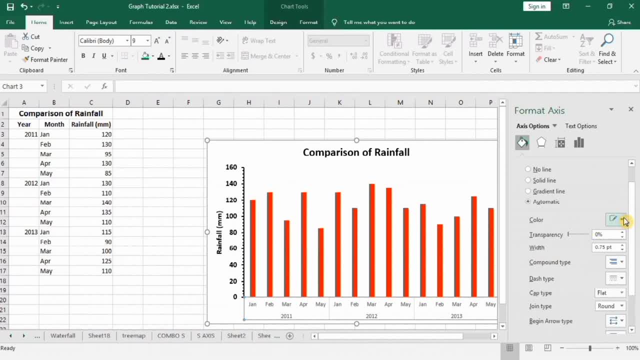 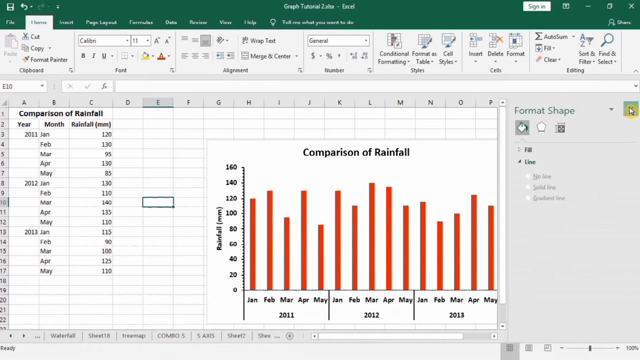 axis, solid line, black color with 1.5 and adjust its color and font size. Now we have formatted a little bit, but the graph look is not desirable, So select these bars by clicking on any bar, right click. go to format data series and 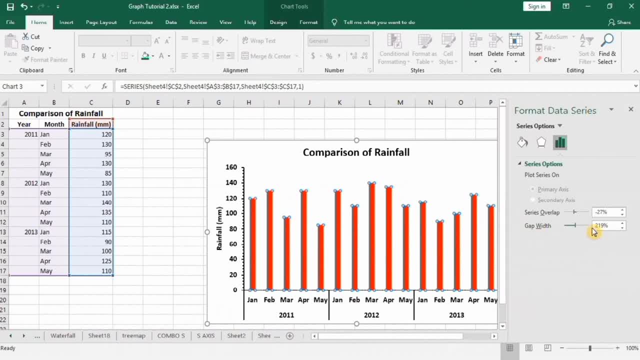 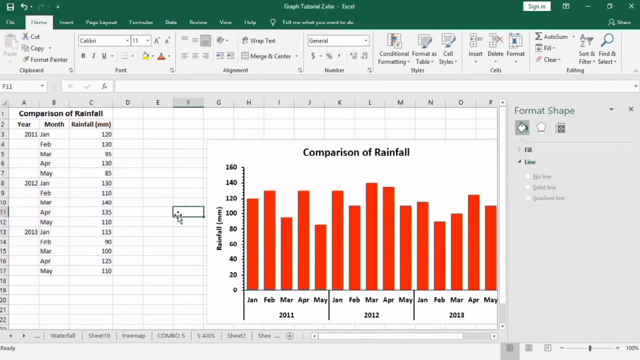 in gap width. you can adjust the gap width to 50%. you can use this option or up and down arrow, but the easiest one is the right here, directly 50.. Now I want to insert the gap between these categories so it is clearly visible. select. 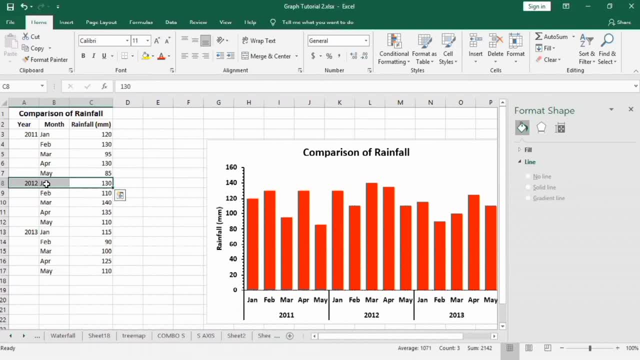 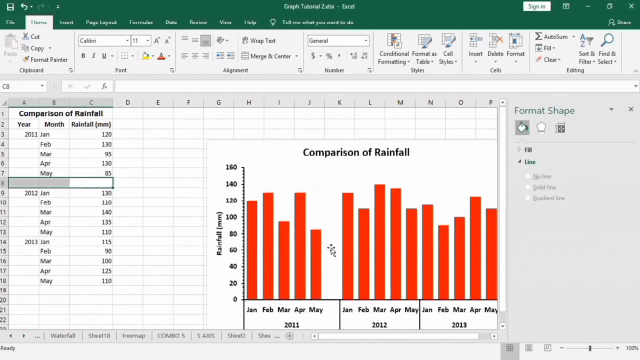 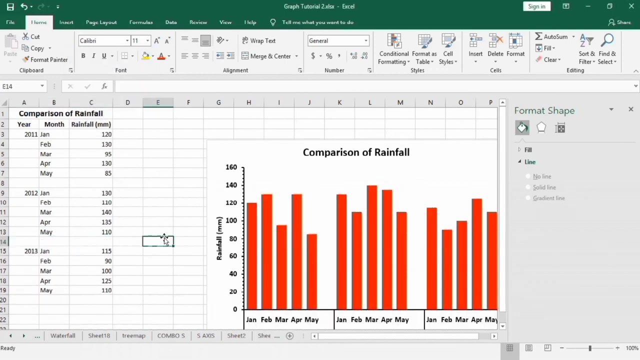 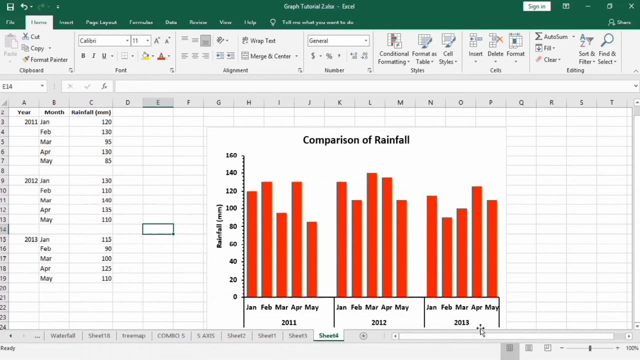 this one: right click and insert entire row. click on ok. you can see here. gap is visible. now Similar step for this one: Click on ok. Right click, go to insert entire row and ok. Now you can see here that the label which appeared here is not at center, exact center. 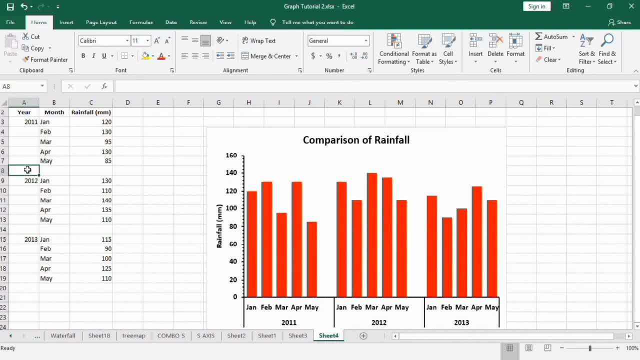 So I will select this one and press space button. Similarly, select this cell First one and press space button. Now select these all columns And change their color. Right click, go to the top of the column, Select this one and press space button. 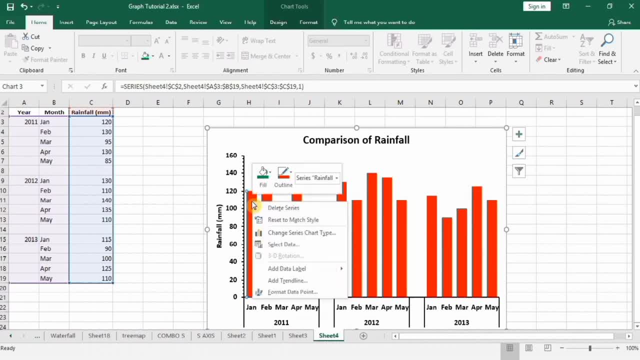 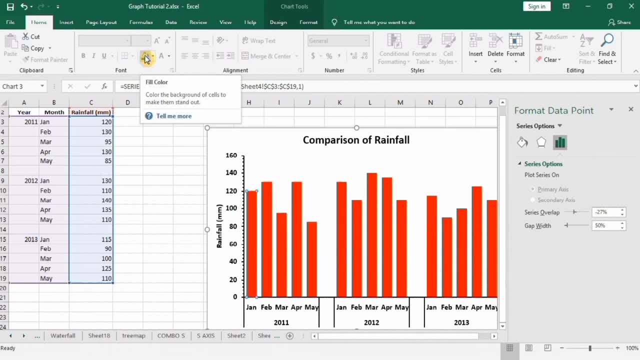 Now select these all columns And change their color. Right click go to insert. Select this one and press space button. Right click format data point. So just select here and you can directly format color by using fill color option. Similarly, select this one and if you want to insert border, just like I have showed in,